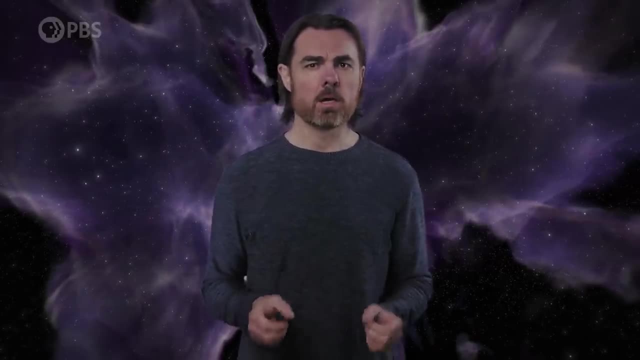 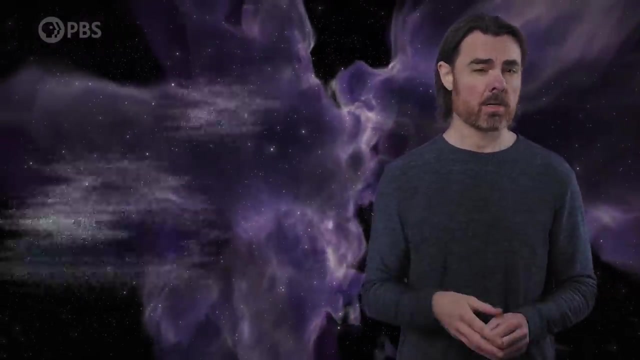 Or at least teach us profound truths about the nature of reality. The trick is going to be to think about mass not as one property of an object, but rather as two distinct and independent properties. There's inertial mass, the resistance to being shoved or slowed. 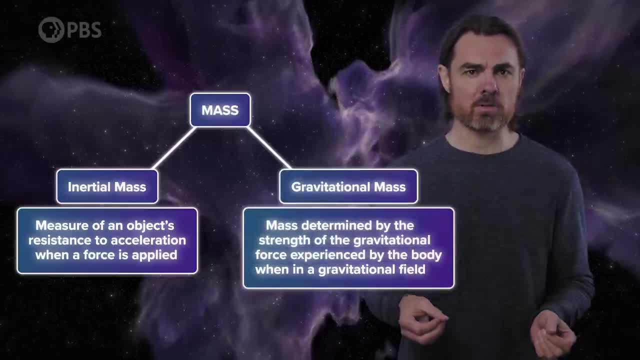 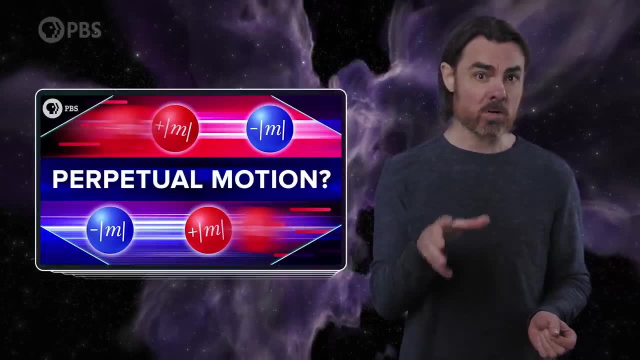 and there's gravitational mass, which determines the heft of your gravitational field and your response to other such fields. Now, we've explored an aspect of this idea previously and this is a good review episode for the studious or a good follow-up episode for the impatient. 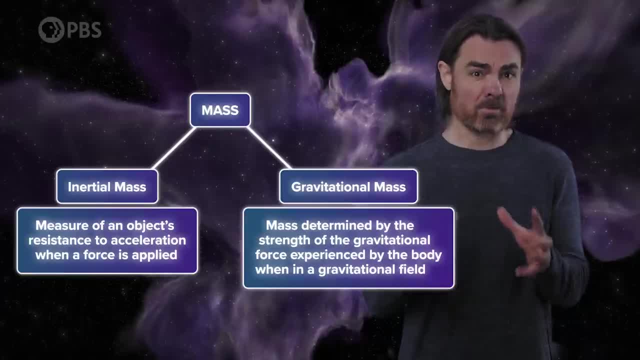 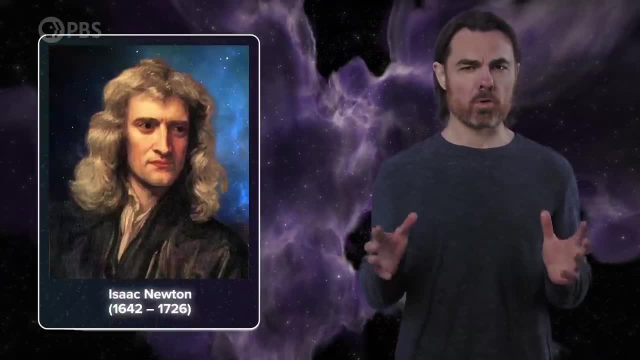 Today we're going to focus on the antimatter and the flying car implications of splitting inertial and gravitational mass. Let's start with Isaac Newton's description of all of this. We'll move to Einstein's upgrade later. Inertial mass is the mass in Newton's second law. 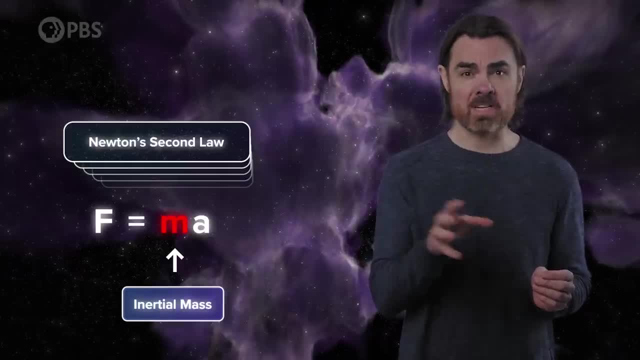 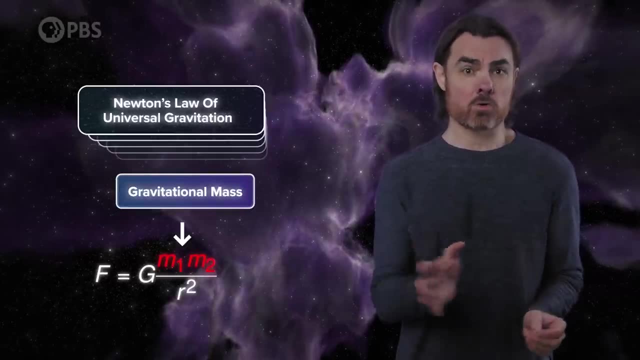 It determines how much force you need to apply to achieve a given acceleration. On the other hand, gravitational mass- the mass in Newton's law of universal gravitation- It acts as the gravitational charge determining the strength of the gravitational field and the strength of response to another such field. 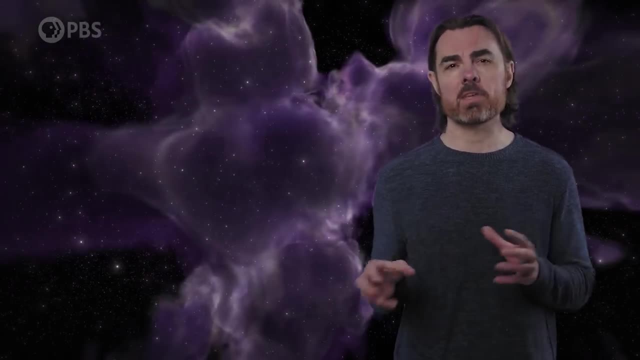 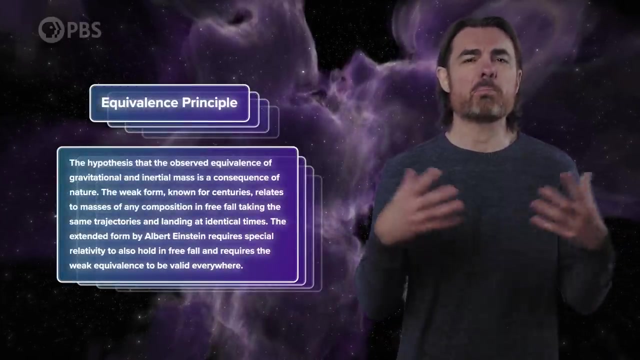 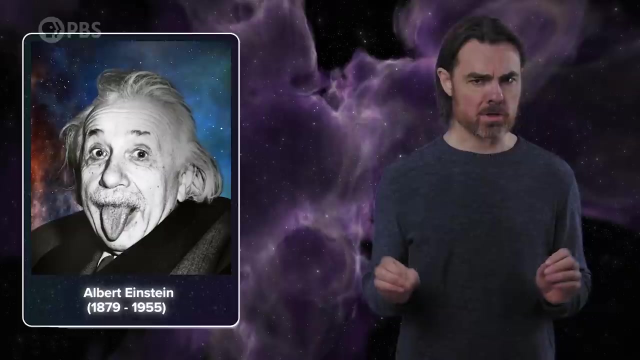 We almost always assume that inertial mass and gravitational mass are the same thing. This equivalence is called the equivalence principle. We normally think of the equivalence principle as being the epiphany that led Einstein to the general theory of relativity, but it's older than that. So a hundred years ago Einstein realized that there should be no 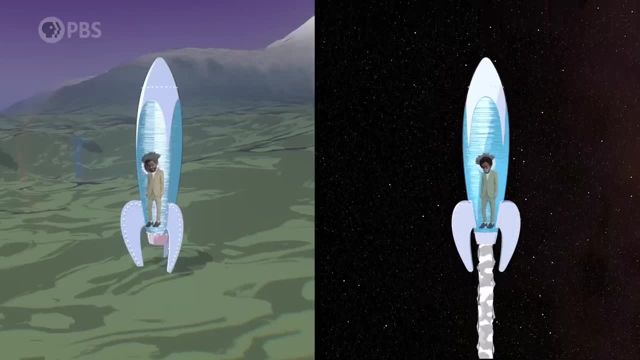 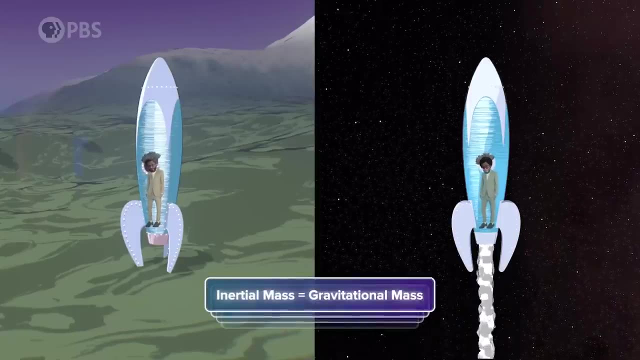 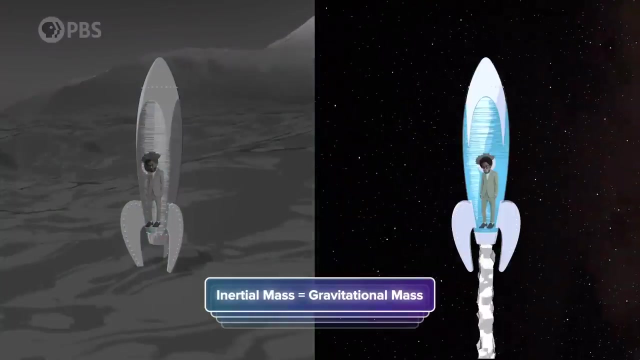 experiment that could distinguish between the feeling of weight you have when supported in a gravitational field and the same feeling when being accelerated at the correct rate in empty space. This statement of the equivalence principle requires that inertial mass- the mass resisting acceleration, is the same as gravitational mass, the mass that responds to a gravitational field. 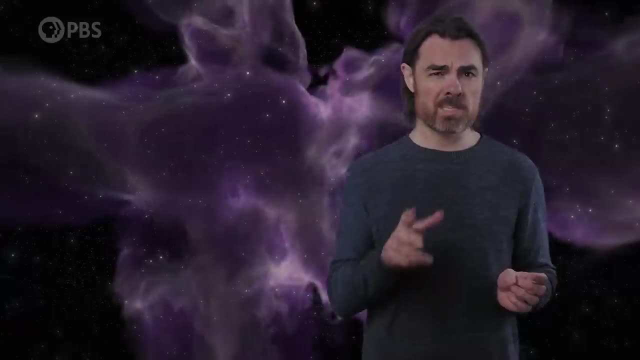 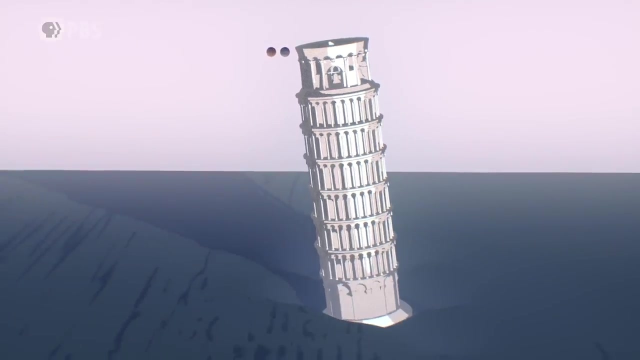 But over 300 years prior to Einstein, this guy named Galileo demonstrated the same thing when he dropped a pair of balls off the top of the Tower of Pisa. They had different weights but the same size, so their air resistance was equal. He found that 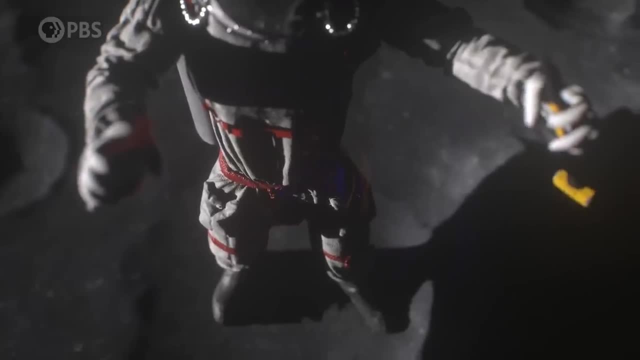 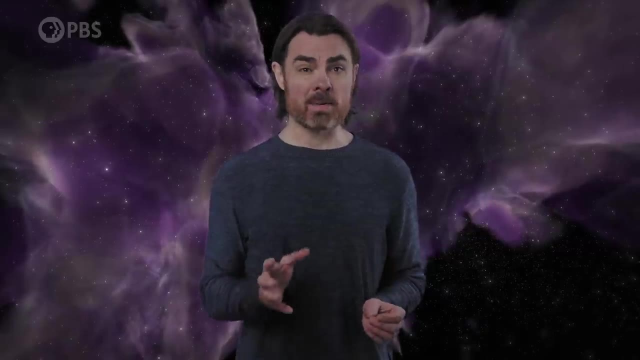 they reached the ground at the same time. We have now done this experiment in the near vacuum of the moon's surface, with a hammer and a feather, giving the same result. Around a century after Galileo's Pisa drop, Newton came along and figured out the equations that tell us why. 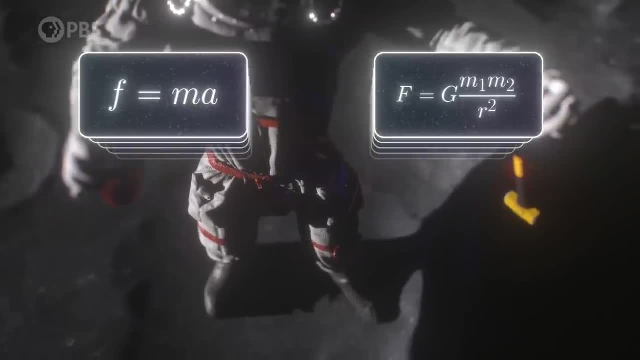 Let's say that the gravitational mass in Newton's gravity law is the same as the inertial mass in the moon's surface. This is the same as the inertial mass in the moon's surface. This is a same as the inertial mass in Lincoln's second law of mechanics. 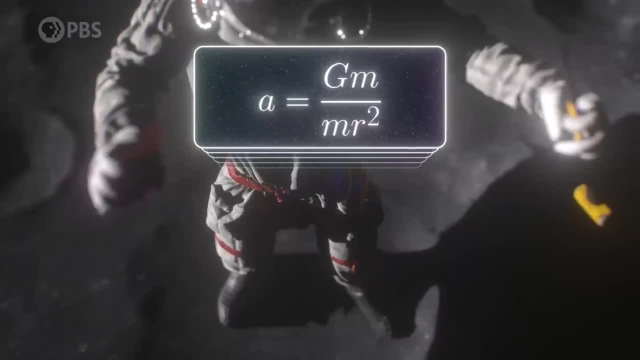 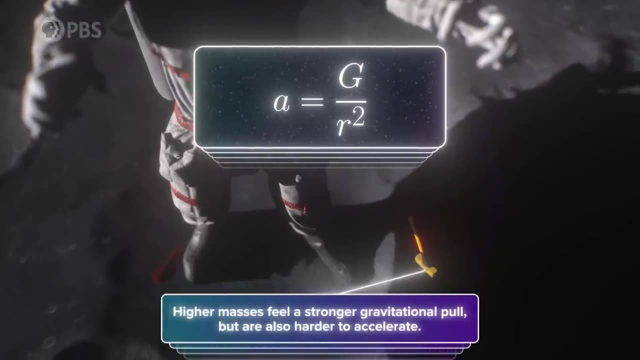 Then, when we calculate the acceleration experience by a massive object in a gravitational field, these two masses cancel out. In other words, more massive objects feel a stronger pull but are also harder to accelerate. Because of this. hammers and feathers fall at the same. 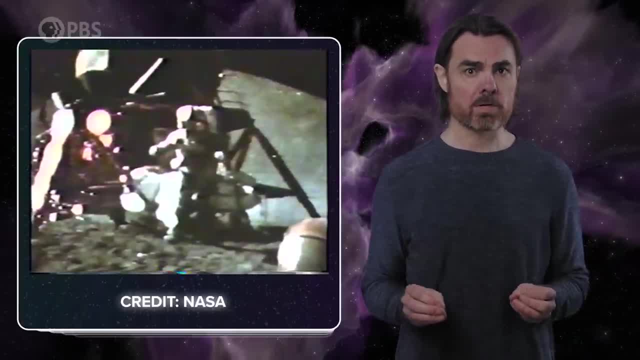 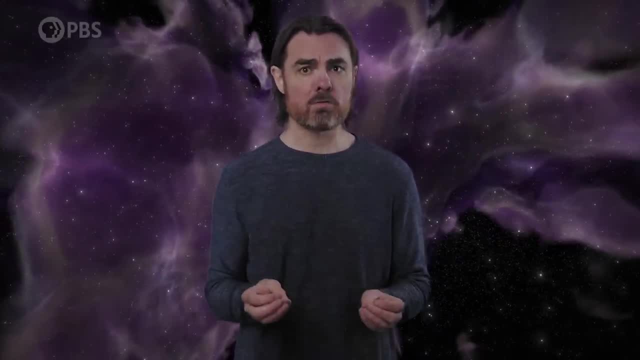 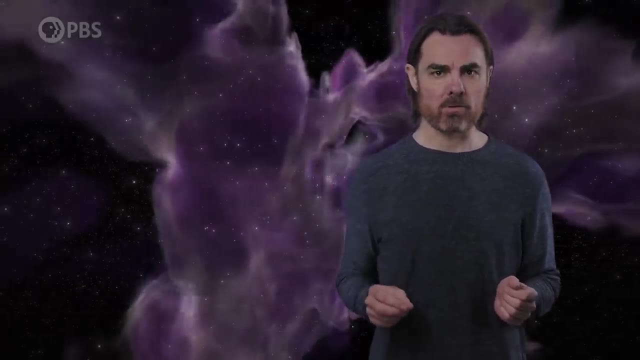 rate on the moon. Gravity is always attractive because gravitational charge, aka mass, is always positive, Compared to electromagnetism, which can be attractive or repulsive due to electric electric charge being positive or negative. So what happens if we allow mass to be positive or negative? 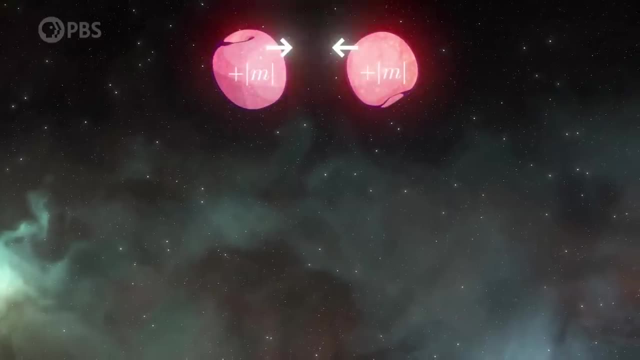 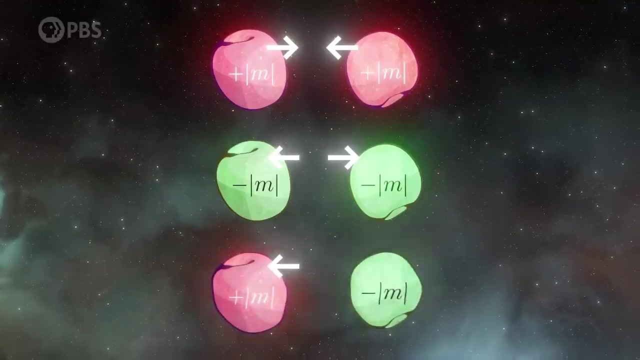 We covered the details in our previous video, but long story short is that two positive masses behave as normal, two negative masses repel each other and a positive mass is repelled by a negative mass, while the negative mass is attracted to the positive. 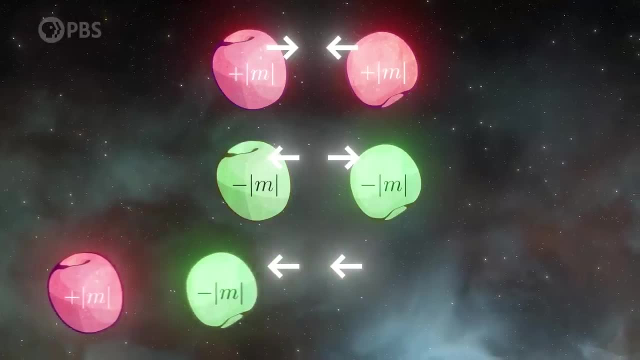 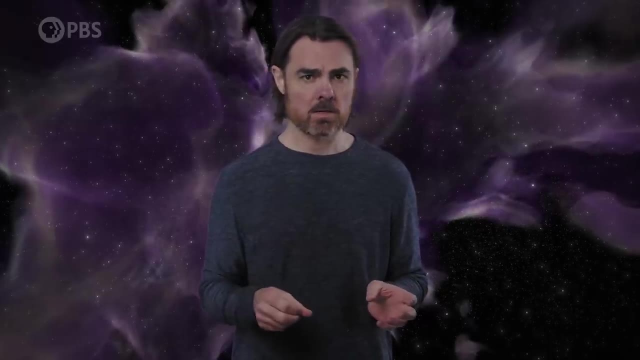 That last part means positive and negative mass would chase each other, accelerating at a constant rate forever. That breaks conservation of momentum and energy, and so can't be right. The thing that really breaks physics in this scenario is that we allow negative inertial. 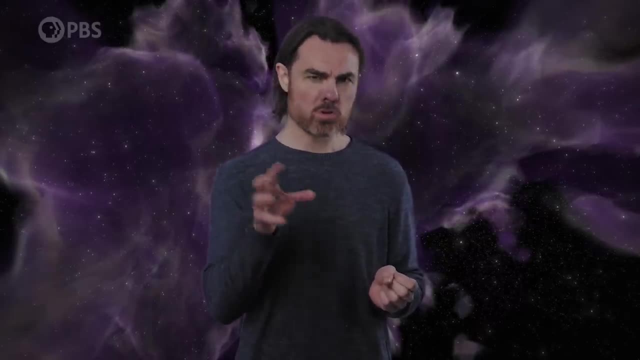 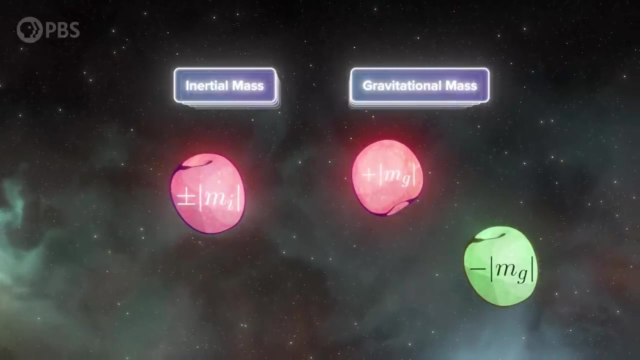 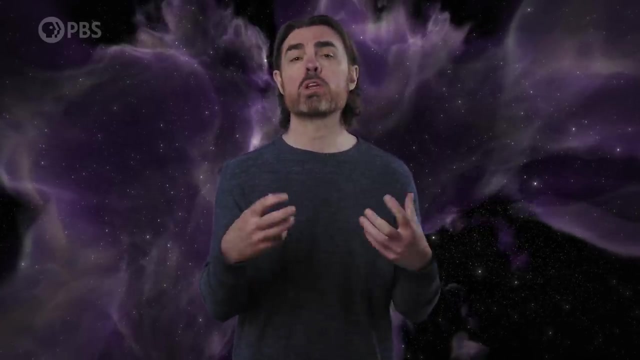 mass, which will always move in the wrong direction to an applied force. But perhaps we can fix this by separating our mass types. What if inertial mass is always positive but gravitational mass can be positive or negative? Then a pair of positive and negative gravitational masses will mutually repel each other, which 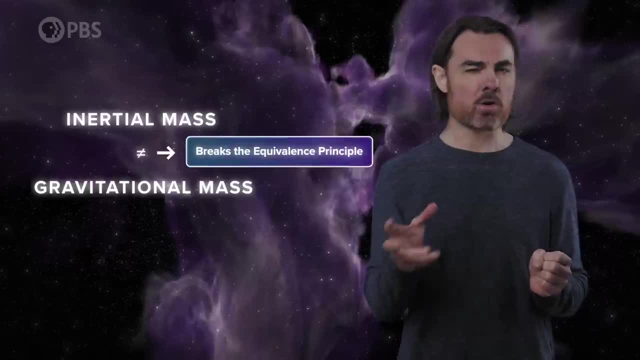 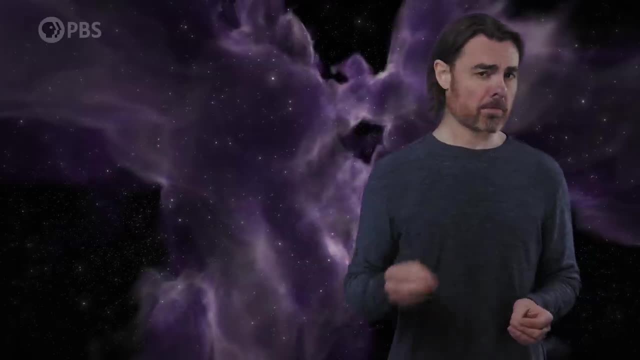 is just what we want. But if we say that inertial and gravitational mass are not equivalent, then we've overturned the equivalence principle. We should not do that lightly. After all, it's one of the founding axioms of general relativity, which is itself an 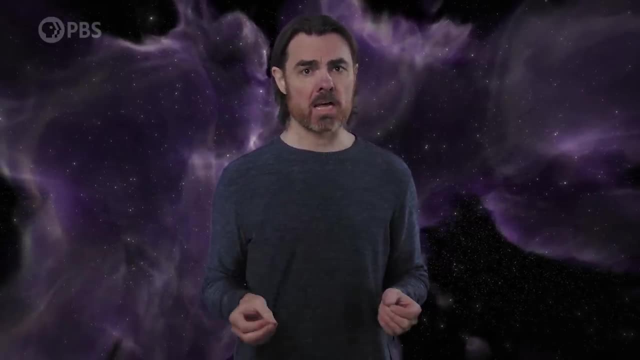 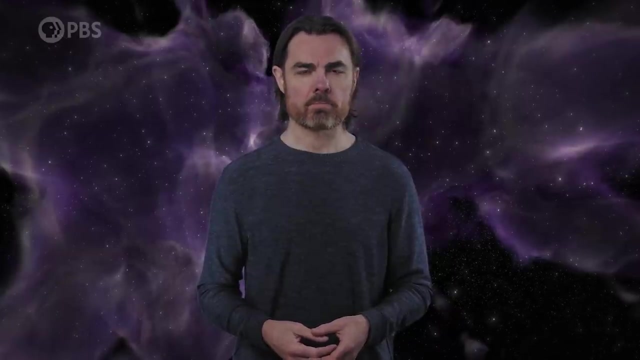 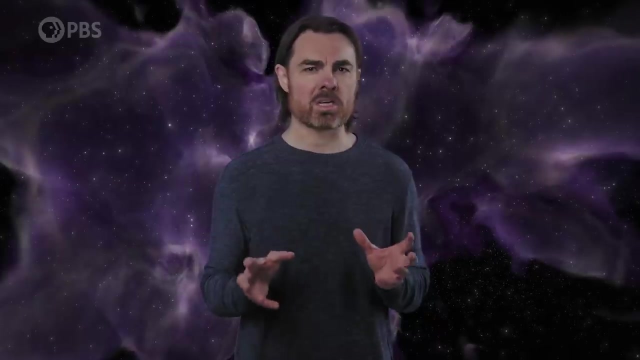 insanely successful theory, But it turns out that, for the type of repulsive gravity that we're looking for, we have to break the equivalence principle. Speaking of general relativity, let's see how negative masses work here. In GR, gravity is explained as mass, causing the fabric of space and time to curve, so 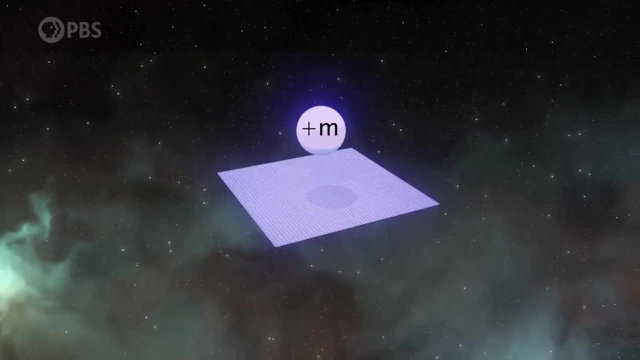 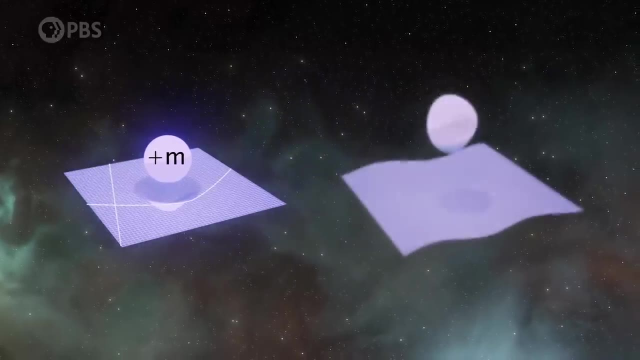 that things move differently due to that curvature. In the classic rubber-sheet analogy, objects with positive mass depress the sheet, causing straight lines to deflect towards them. Hypothetical negative gravitational masses would be depicted by pinching the sheet upwards, causing straight lines to move away. 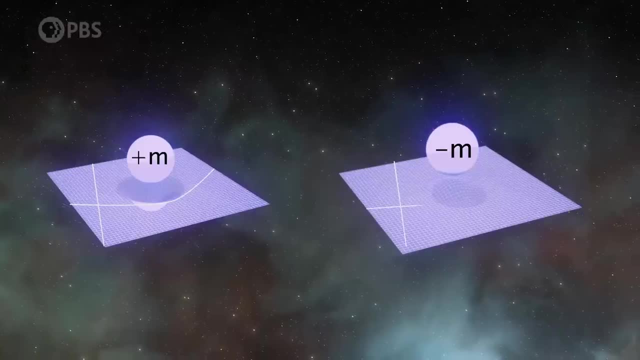 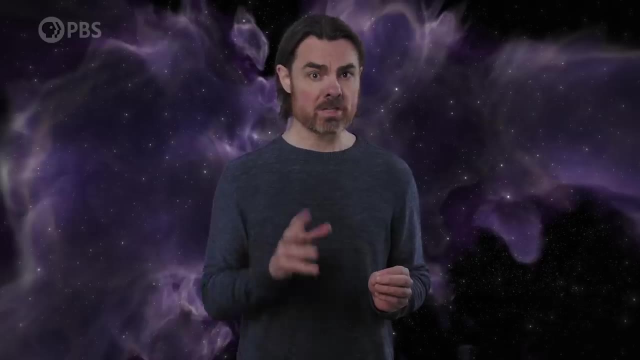 This picture makes it somewhat intuitive why the motion of particles seems to only depend on the shape of the gravitational field, which itself depends only on the gravitational mass of the central object. Objects follow, geodesics, the straightest lines in curved space, regardless of their 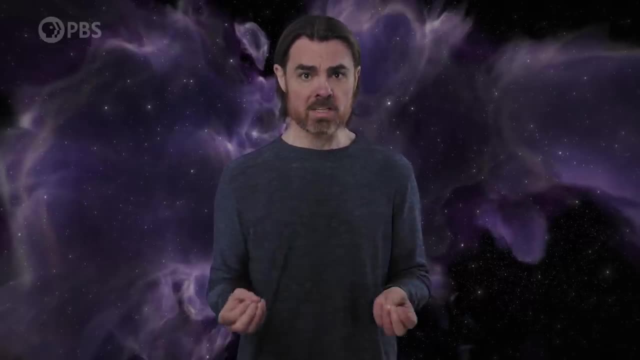 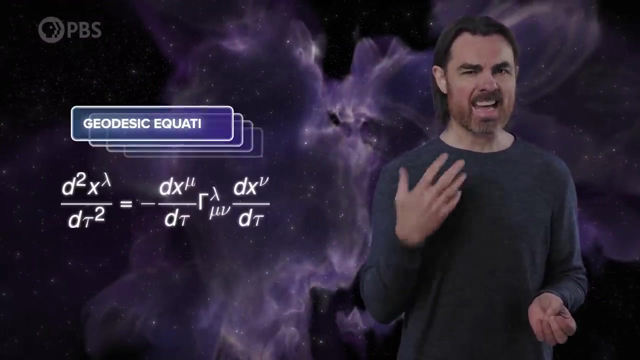 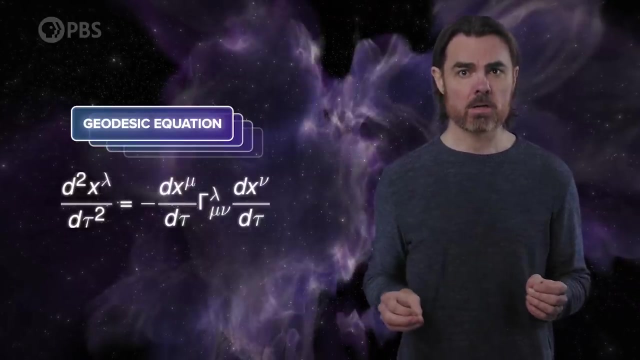 own mass. In fact, we can also think of this as the gravitational and inertial masses cancelling out, just like with Newtonian gravity. We can see that cancelling in something called the geodesic equation, which is the equation of motion for a particle in general relativity. 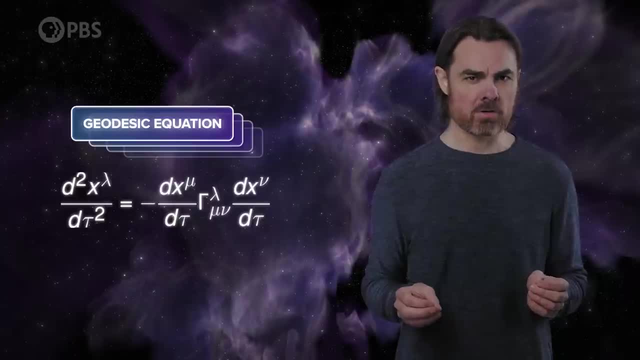 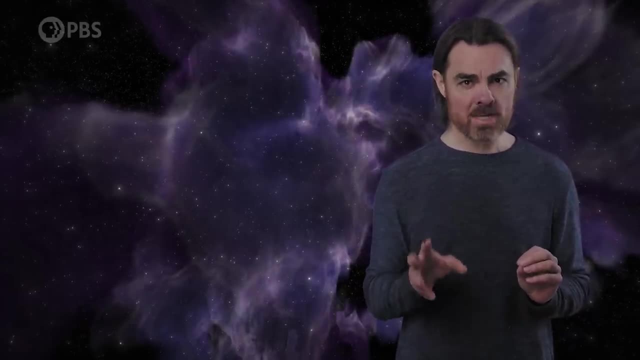 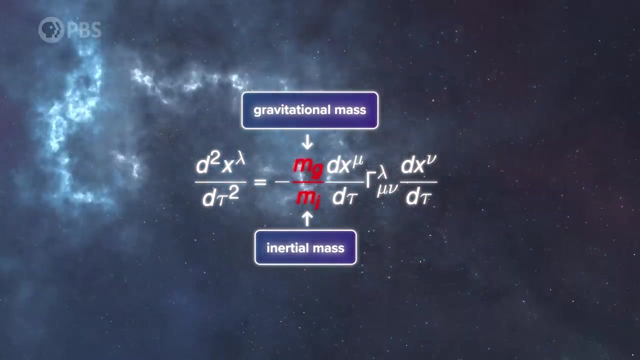 Normally the mass of the moving object doesn't appear in this equation, just like it doesn't in the Newtonian acceleration equation, But it's actually hidden If we separate inertial and gravitational masses. we see it here, And the geodesic equation also tells us how positive and negative gravitational masses 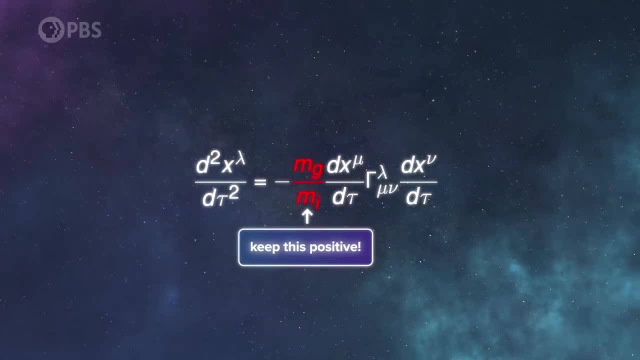 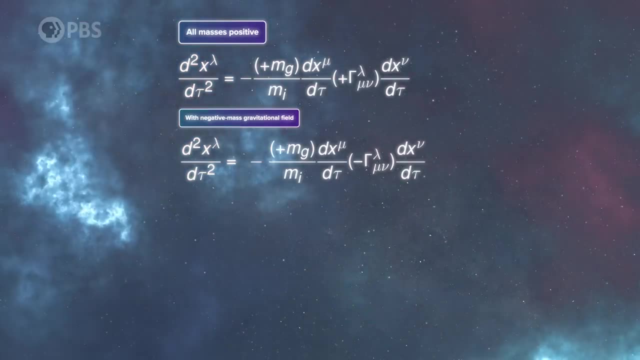 interact. We're going to keep inertial mass positive, because anything else is insane. Now, negative gravitational masses change the sign of the gravitational field or the sign of the mass of the interacting particle, or both, If both masses are positive or both negative. 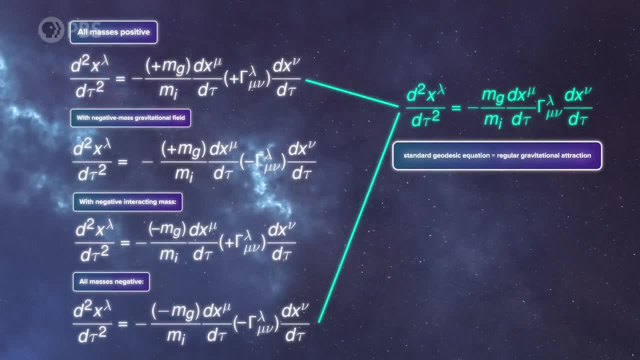 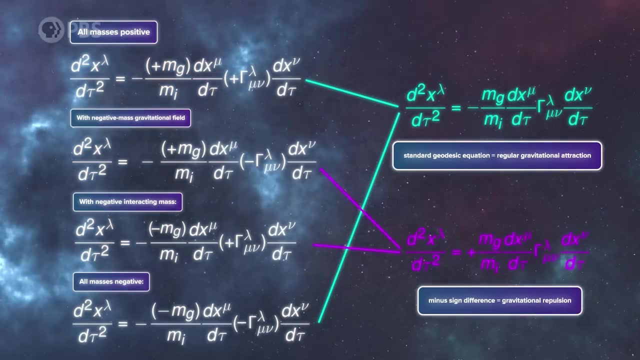 If both masses are positive or both negative. If both masses are positive or both negative, The minus signs get cancelled and we have regular gravitational attraction. But if only one of those masses is negative, then we end up with a new minus sign between the field and the object. 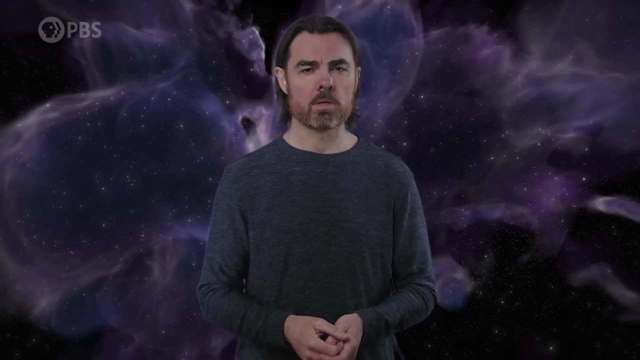 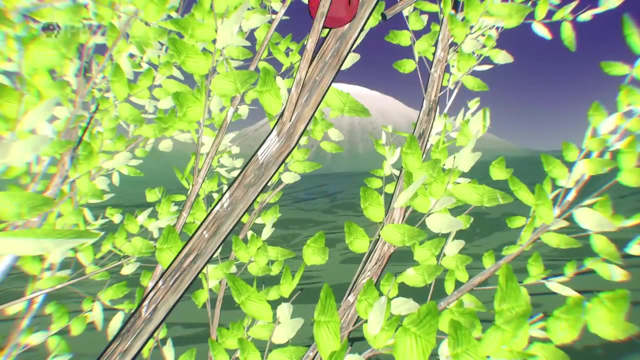 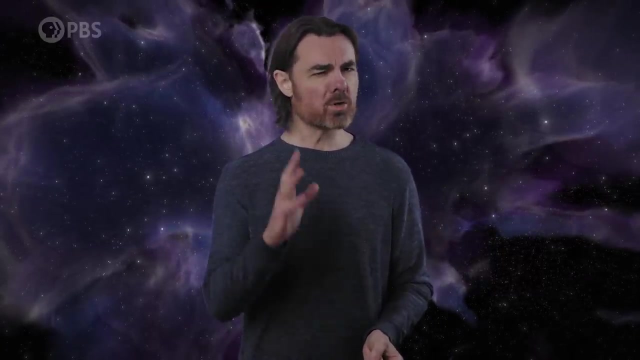 The effect is gravitational repulsion. In other words, something with a negative gravitational mass would fall upwards in Earth's gravitational field. Okay, great. So to make an anti-gravity engine, we just need a negative gravitational mass. So what's all this about anti-gravity? 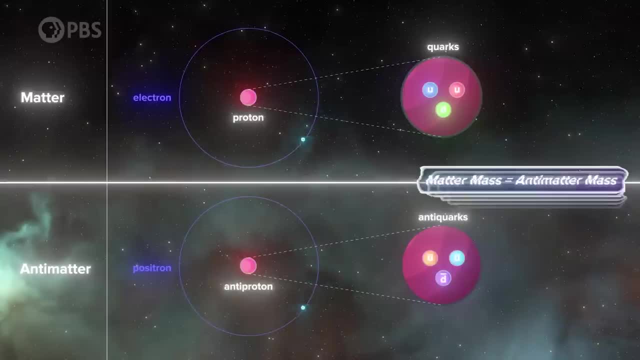 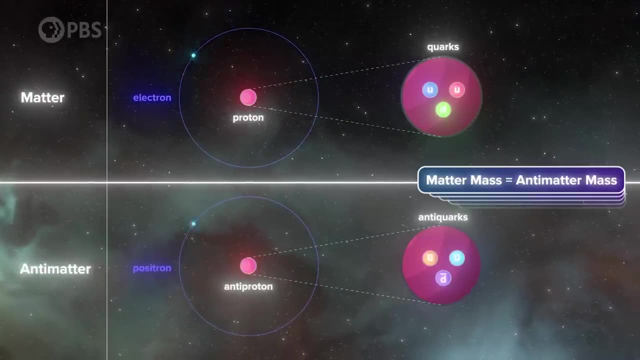 What's anti-matter possibly having this property, An anti-matter particle has the same mass as its regular matter counterpart, but is opposite in many quantum properties, And that doesn't sound helpful. If anti-matter has the same mass as regular matter, then where's our negative mass? 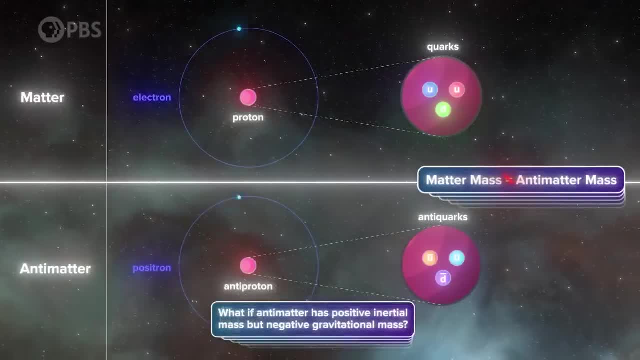 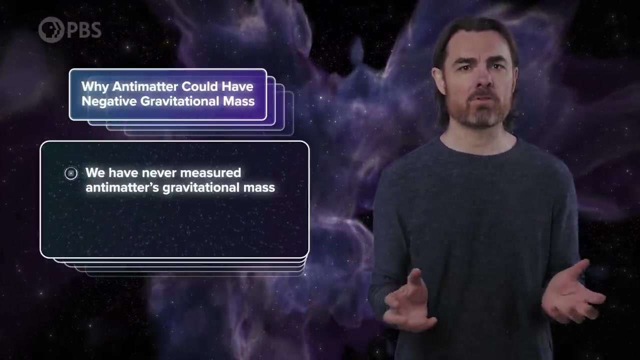 Well, remember, we just broke the equivalence principle, at least in our imaginations. So maybe anti-matter can have positive inertial mass but negative gravitational mass. Two reasons we might think this is the case. First, based on its response to the electromagnetic field, we know that anti-matter does have positive 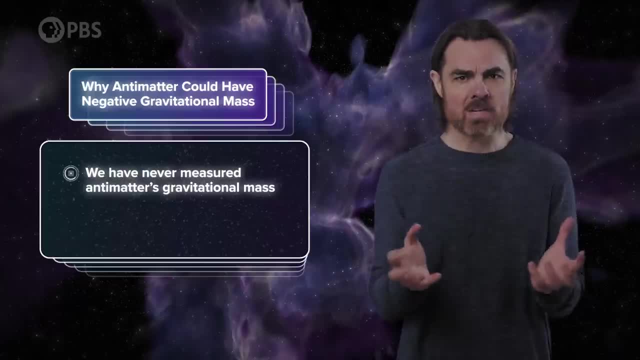 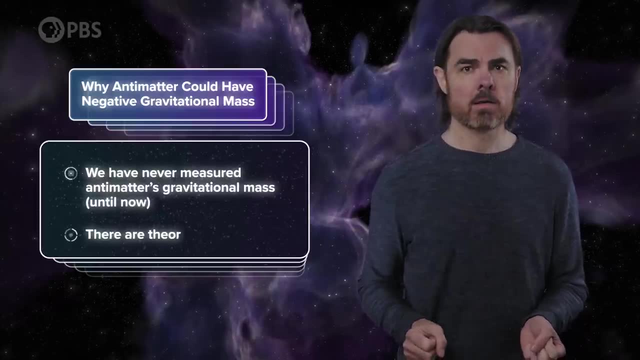 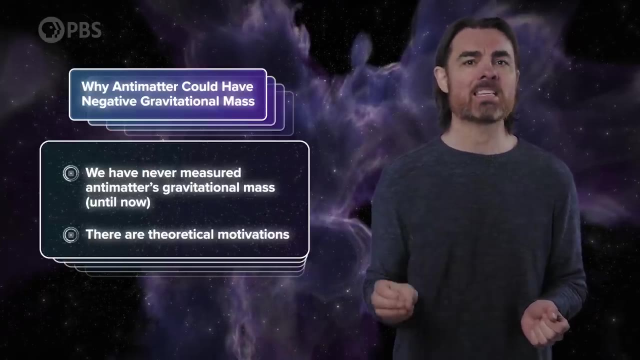 inertial mass, But we've never actually measured its gravitational mass. Well, actually just recently we finally did, and I'll tell you the results in a bit, But we've had a lot of years to come up with. reason two, That there are theoretical motivations for thinking that maybe anti-matter has negative 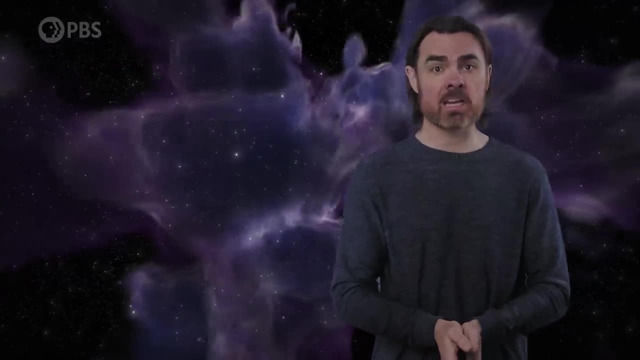 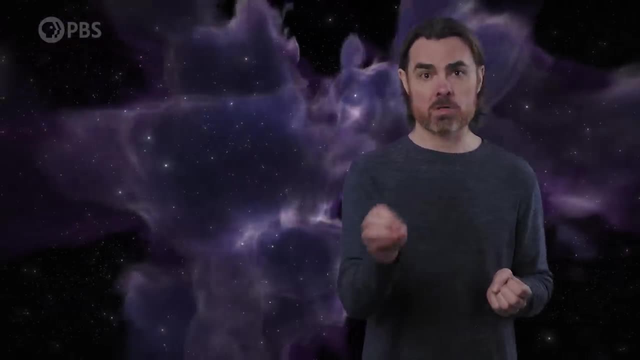 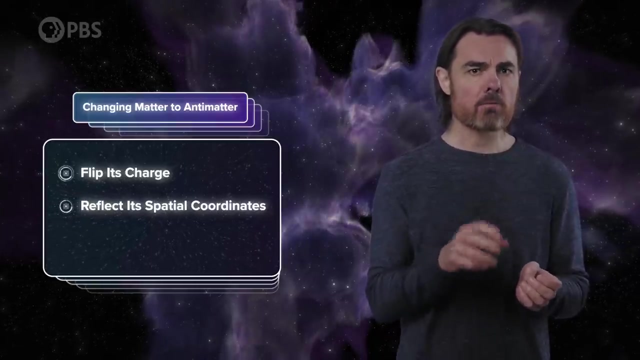 We need to understand the theory behind anti-matter. Anti-matter is what you get when you take regular matter and do three things to it: Flip its charge, reflect its spatial coordinates, so clockwise particles become counterclockwise, and reverse its time axis, which is equivalent to reversing all of its motion vectors. 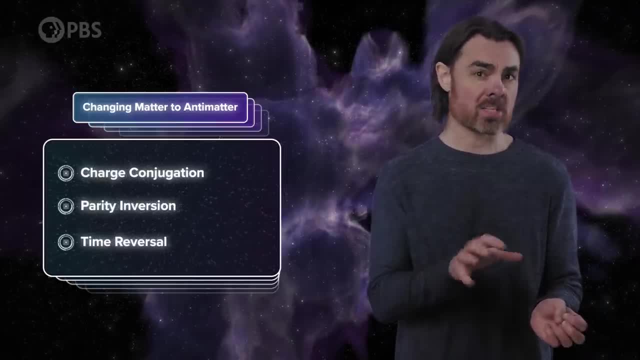 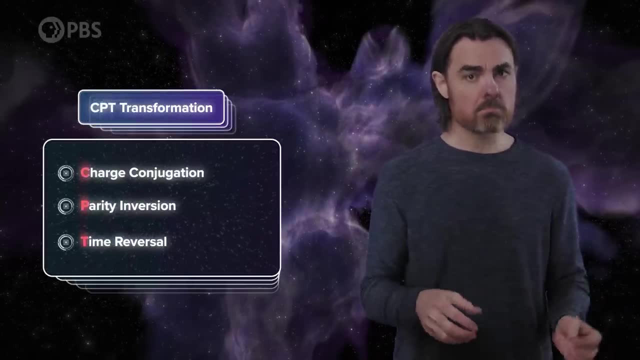 These transformations are called charge conjugation, parity, inversion and time reversal And applied together we have a CPT transformation. CPT transform regular matter and it becomes anti-matter. And of course, there's a homework episode for you on this topic. 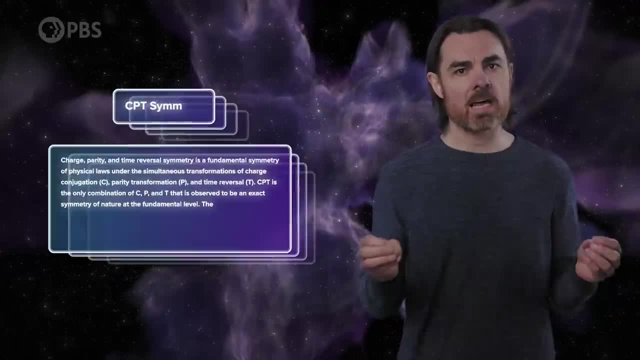 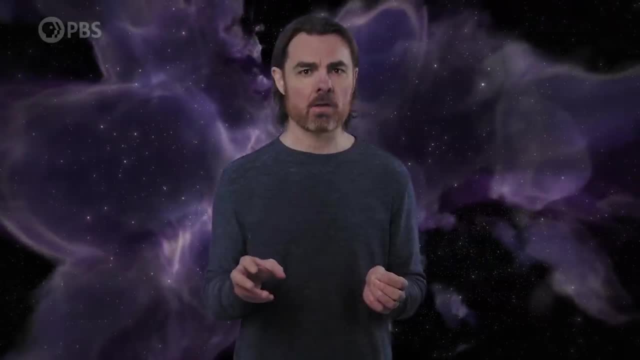 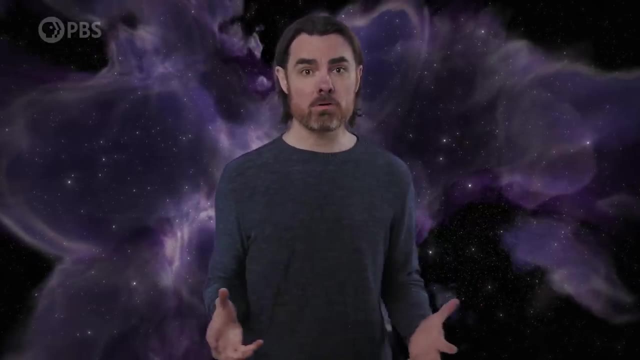 Most physicists think that our universe has to be CPT symmetric, which means that although the laws of physics change, if you perform any of these transformations separately, if you perform all three together, the laws of physics should look exactly the same. CPT transform the whole universe and you get an anti-matter universe that follows exactly. 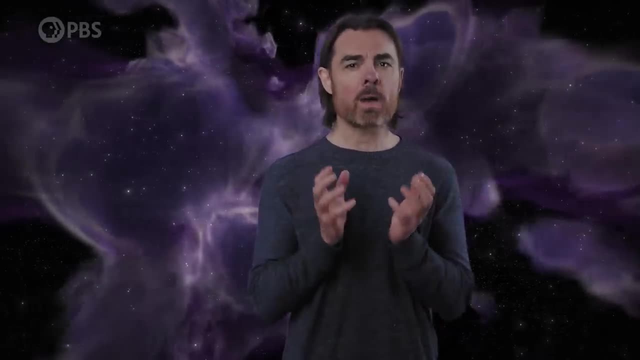 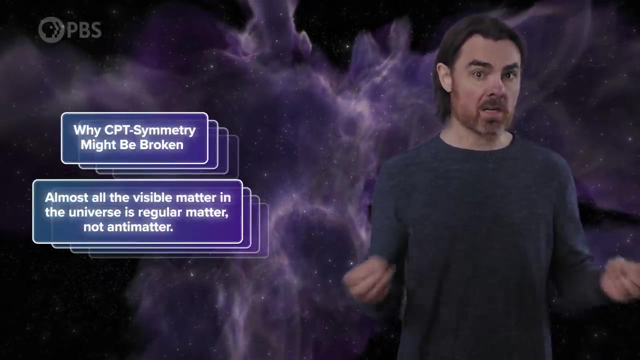 the same laws of physics as our regular matter universe. But there's at least one big reason to wonder if CPT symmetry is broken, Why? And that's because almost all of the matter in the universe is regular matter with hardly any anti-matter. 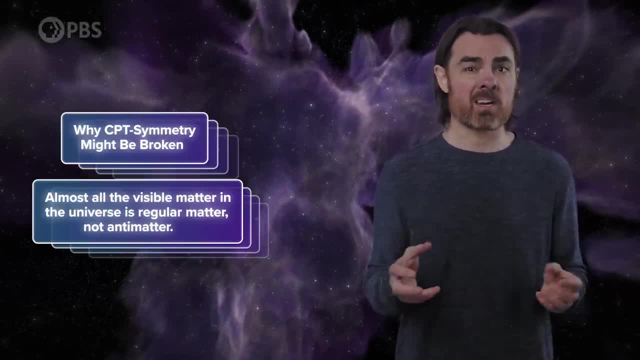 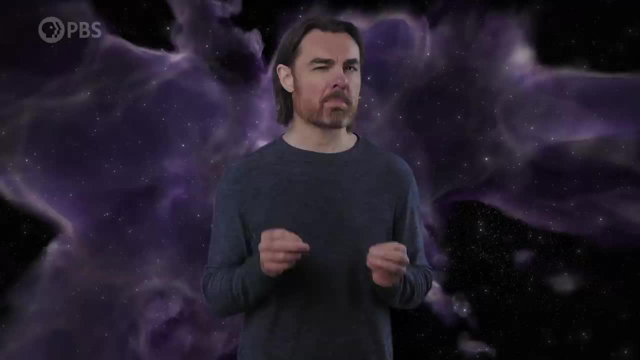 In a perfectly CPT symmetric universe, matter and anti-matter probably should have been created in equal quantities soon after the big bang. If we found out that CPT symmetry is broken and how it breaks, we could perhaps solve this big mystery. 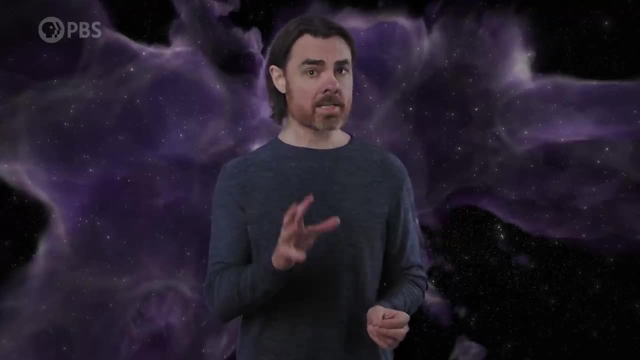 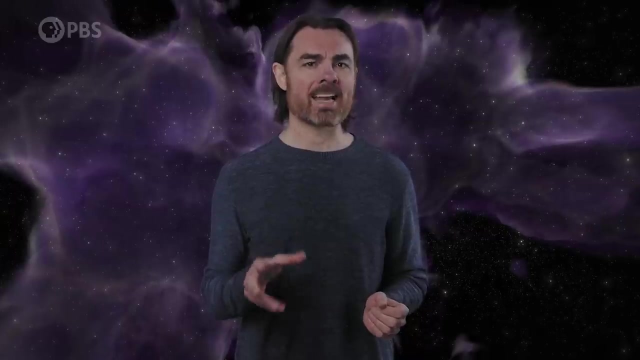 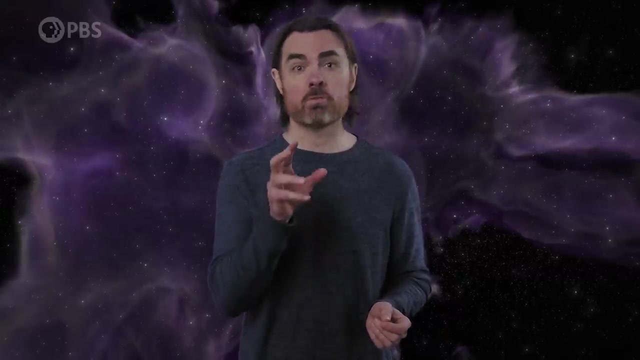 But I digress. We are here to build a flying car, And understanding the CPT symmetry can help us do that. If this symmetry is true, then… Then all the laws of physics should look the same under CPT transformation. So an anti-matter universe should run by the same equations, including the equations of. 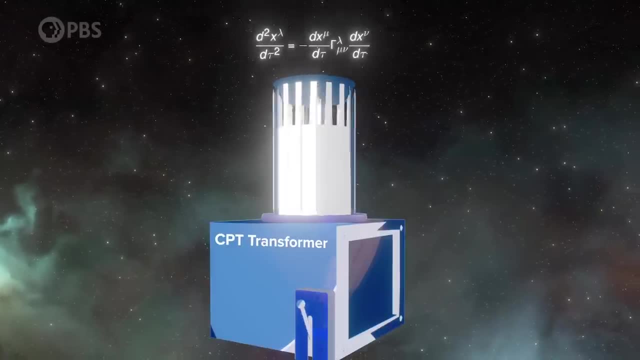 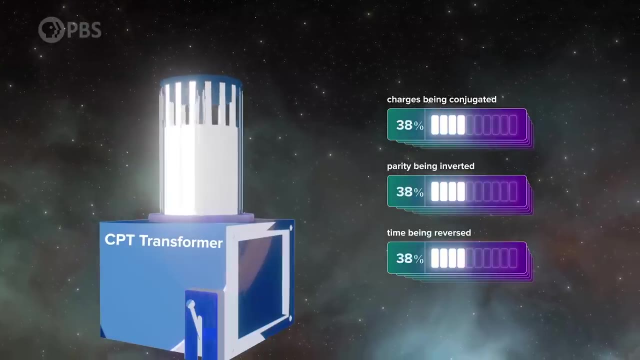 general relativity And indeed if you apply a CPT transformation to the geodesia equation, you'd get some minor signs as you reverse the flow of time and flip the dimensions of space etc. But they cancel out and give you exactly the same equation you started with. 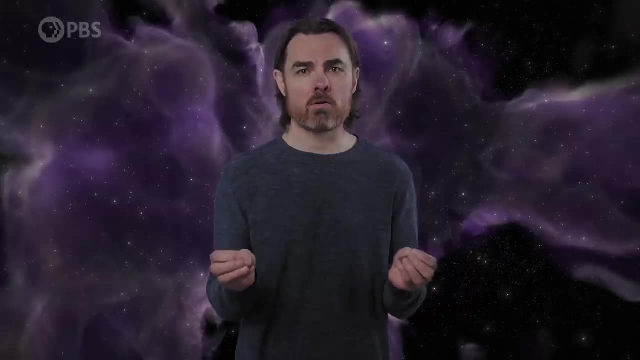 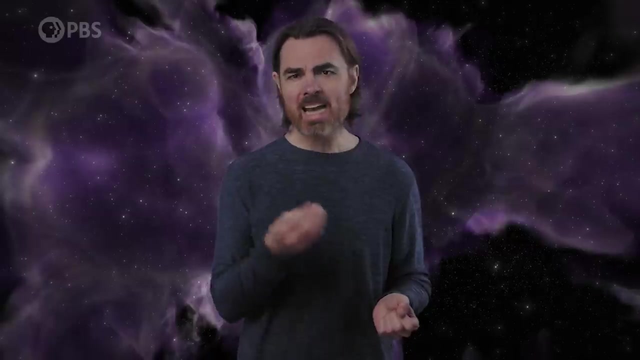 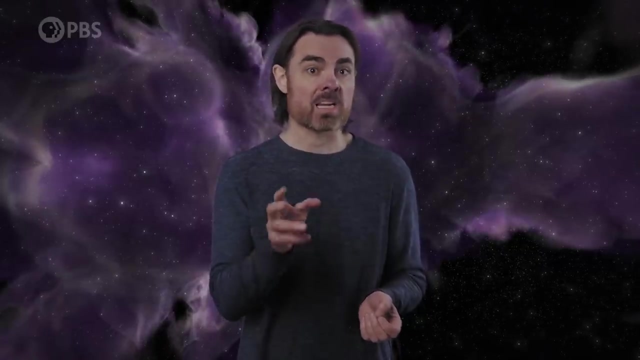 That's equivalent to switching both of a pair of mutually gravitating objects. They'd still attract each other. In fact, we can't even say if they both have positive or negative mass. The math looks the same as long as they have the same sign of mass. 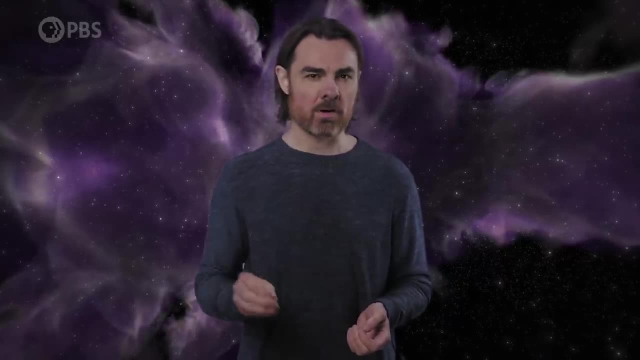 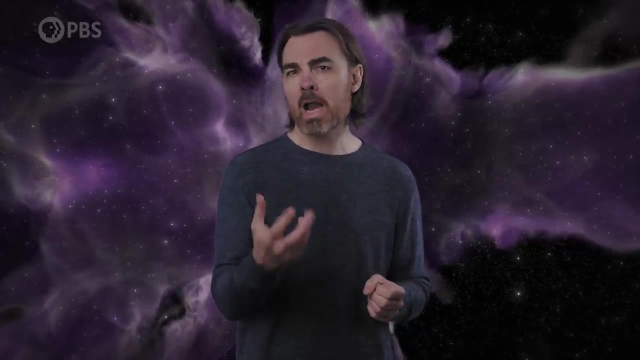 General relativity in general seems to be CPT-invariant. But what happens if you CPT transform only part of the equation, if you turn one of a pair of masses into anti-matter? The exact way a CPT transformation interacts with the geodesia equation is the same as 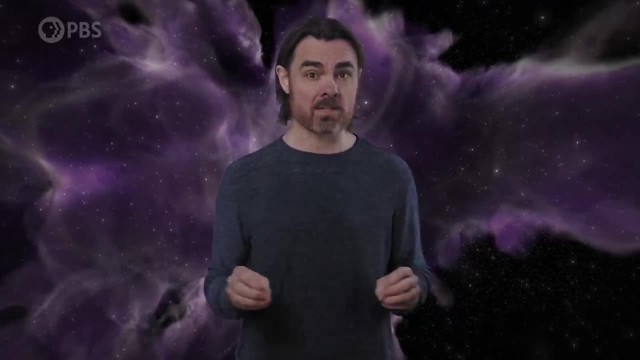 the general relativity. But what happens if you CPT transform only part of the equation, if you turn one of a pair of masses into anti-matter? The exact way a CPT transformation interacts with the general relativity. The exact way a CPT transformation interacts with the general relativity. 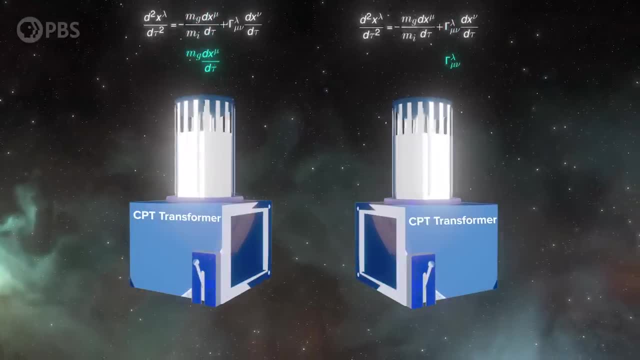 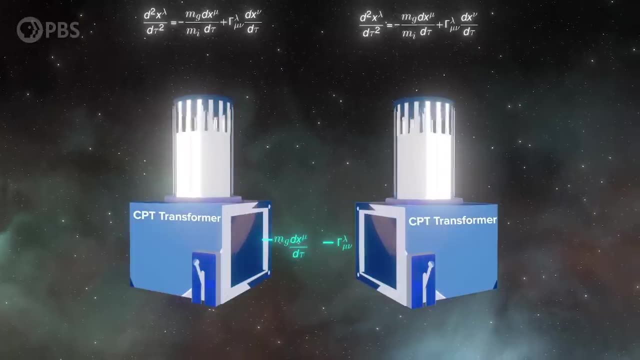 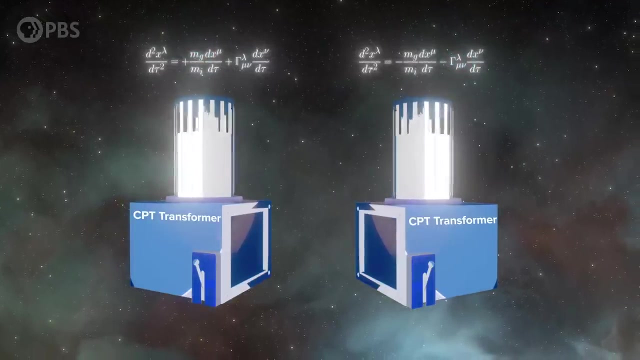 The exact way a CPT transformation interacts with the general relativity. So the result of this equation is to introduce a minor sign to the field or to the mass in motion, depending on which you turn into anti-matter, But mathematically that's equivalent to changing one of the gravitational masses. 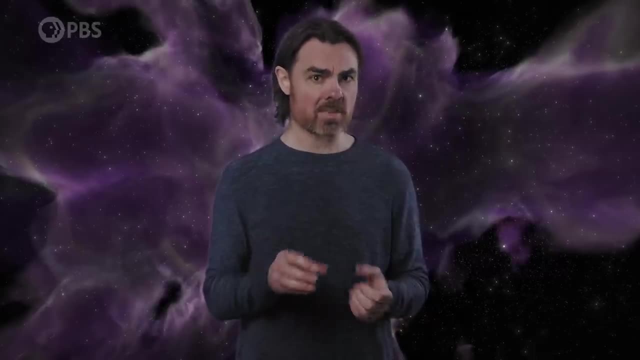 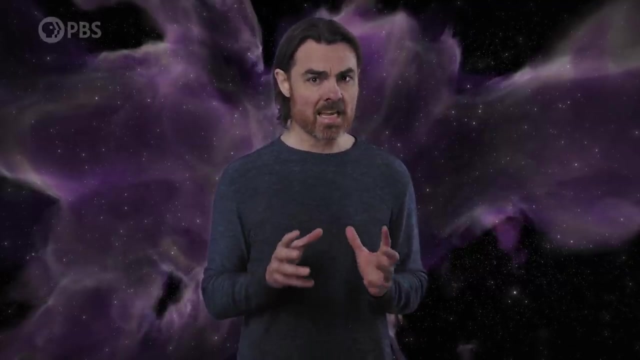 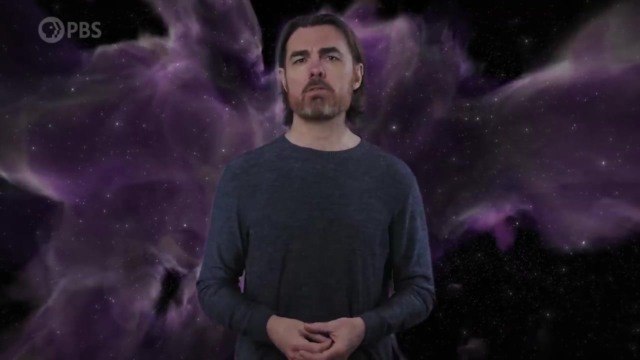 negative. So some ways of thinking about the symmetry of general relativity gives anti-matter negative gravitational mass, Number 5. this is a contested interpretation, but the result would be gravitational repulsion and hoverboards. At the very least, it's definitely worth finding out whether antimatter falls up or down. 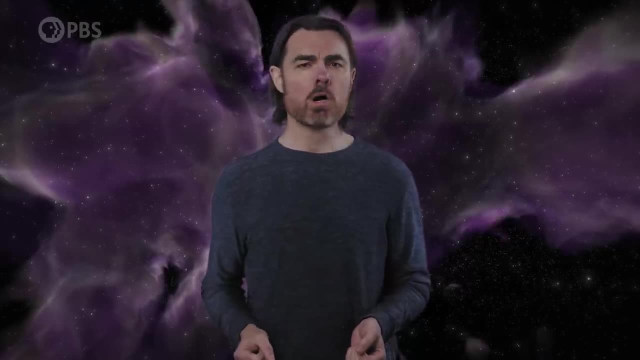 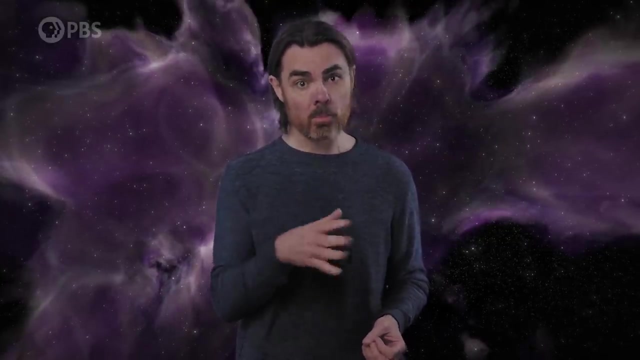 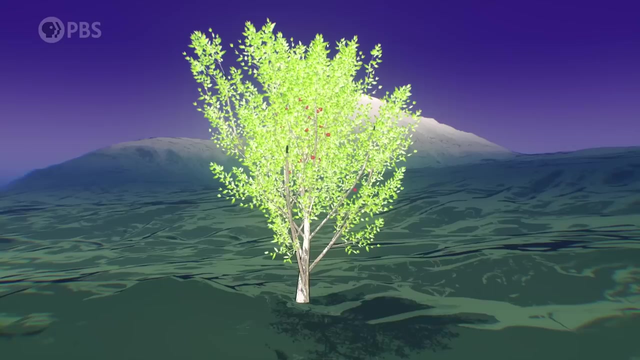 whether for the awesomeness of our vehicular future or just to see if there's any weirdness in the gravitational interaction of antimatter that could poke holes in CPT symmetry and help us answer some very big questions. So let's get to the experiment. Finally, what happens when you? 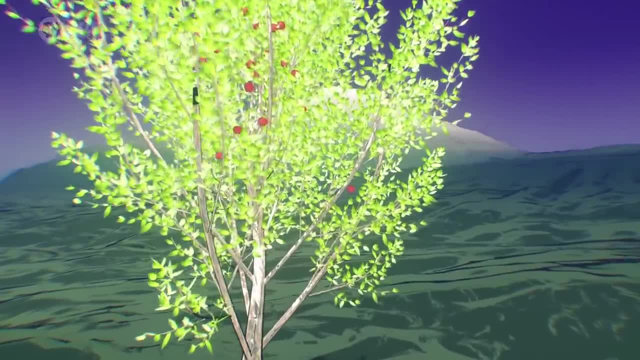 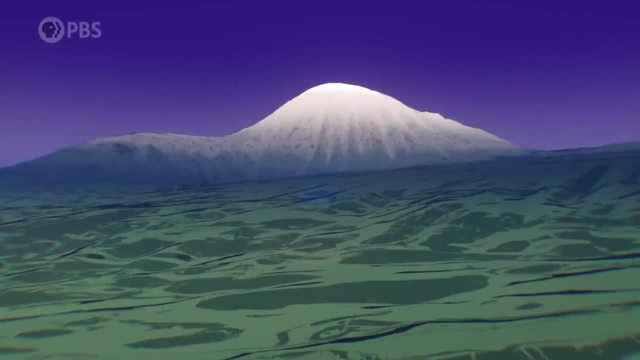 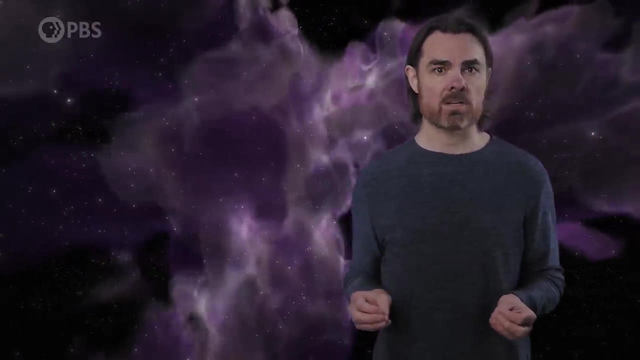 drop an apple made of antimatter And to start with, why is it so hard to even do this experiment? Well, it's because we don't have any antimatter apples. Antimatter is extremely hard to create and to keep contained. It instantly annihilates when it encounters regular matter. At best we have 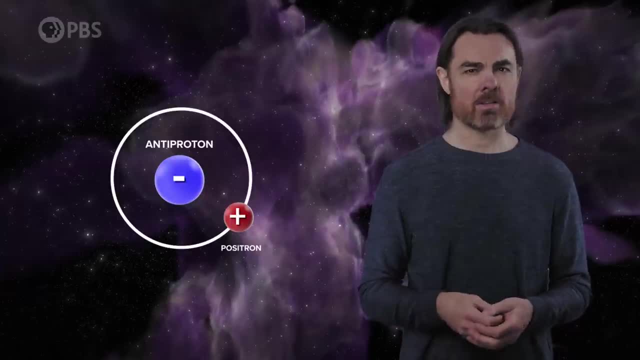 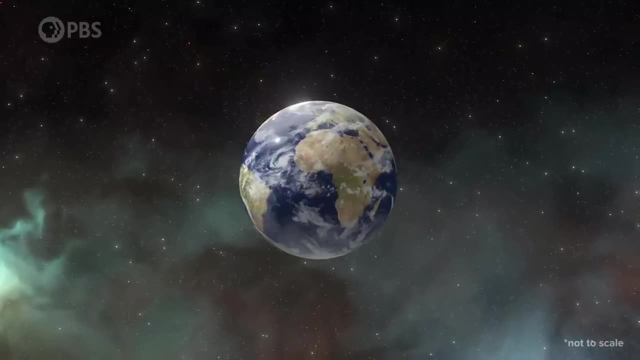 antimatter atoms. The difficulty is also due to the fact that the gravitational force is so weak compared to the other fundamental forces. For example, if we wanted to measure the effects of gravity on a free-fall system, we would need to measure the gravity of a free-fall system. 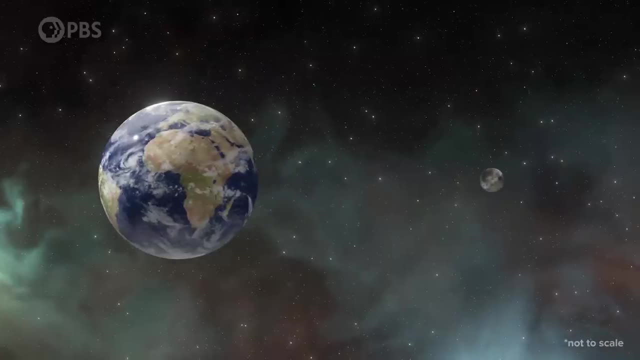 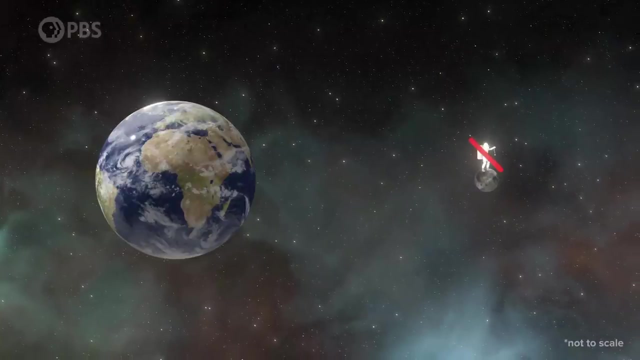 If we had an electron in the Earth's gravitational field, it would be like trying to measure the force of gravity that a human body exerts on a feather- No, not an astronaut's body on the dropped feather, but the force that your body here on Earth exerts on that feather on the moon. 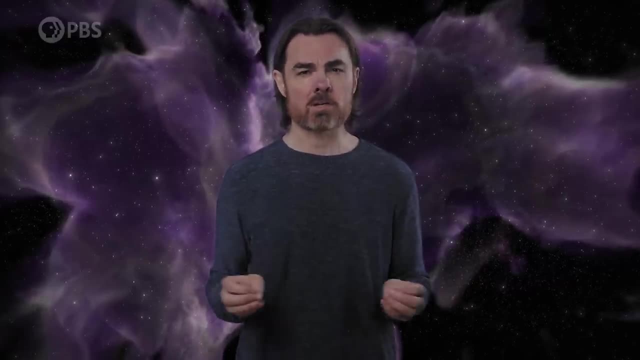 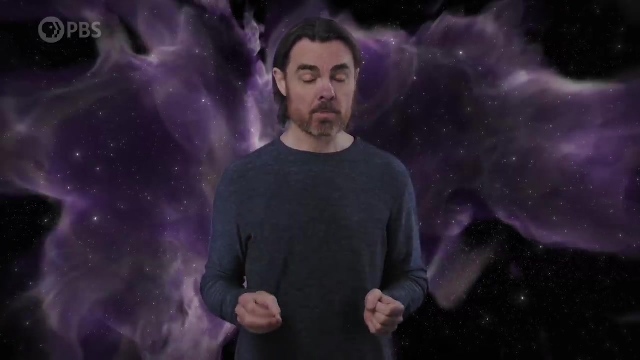 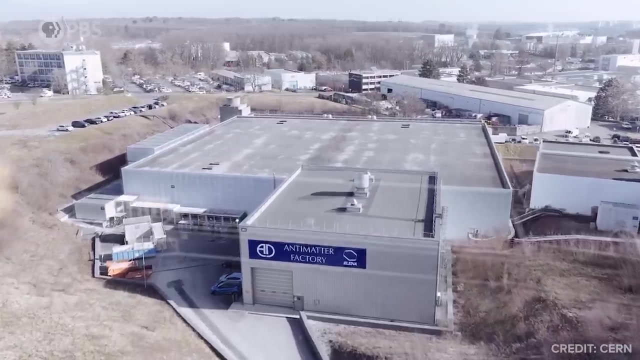 Add the fact that any antiparticle we analyze will be subject to vastly greater forces from ambient electromagnetic fields And this becomes an intensely difficult experiment, but not an impossible one. is a CERN experiment that has been years in the making. It starts with the antimatter. 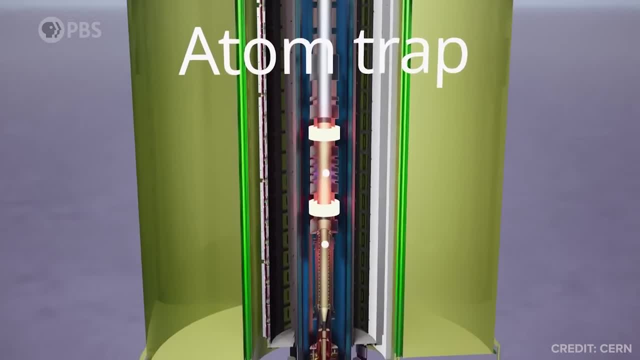 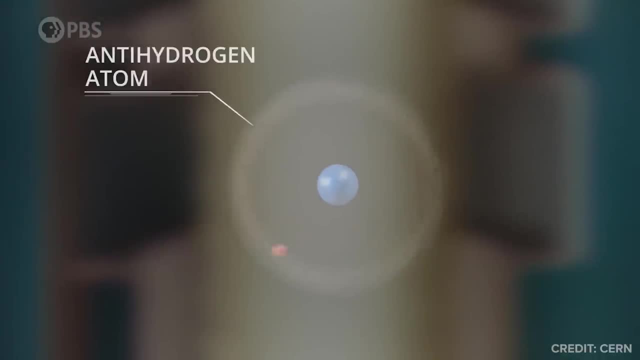 production line by the Alpha Collaboration. This team has managed to create and magnetically trap hundreds of stable anti-hydrogens consisting of a positron orbiting an antiproton. Their sister collaboration, Alpha G, then takes these atoms and drops them in freefall in. 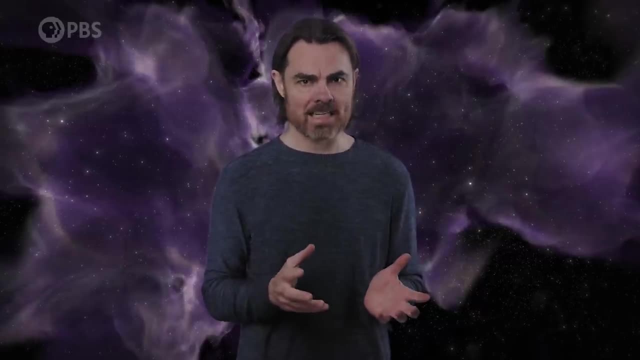 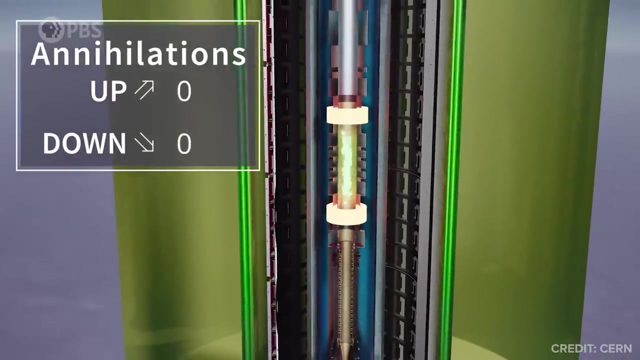 a vacuum chamber. That sounds simple, but it's an extremely delicate operation Because of the extreme smallness of the gravitational force on these atoms and the other effects that jostle them around. they don't all just tinkle downwards, Some move up, some move. 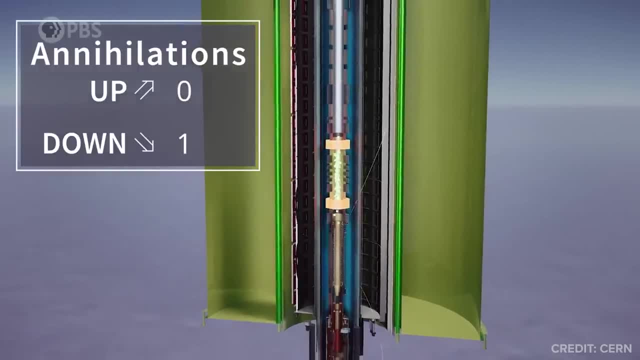 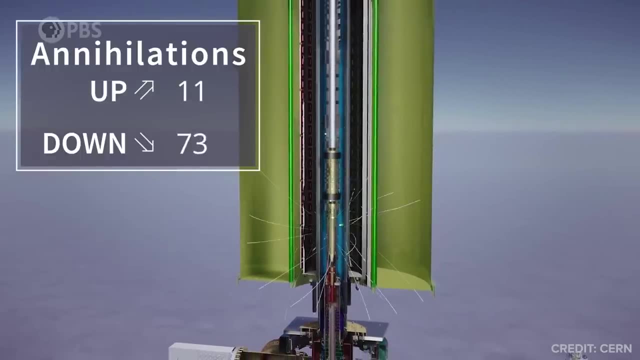 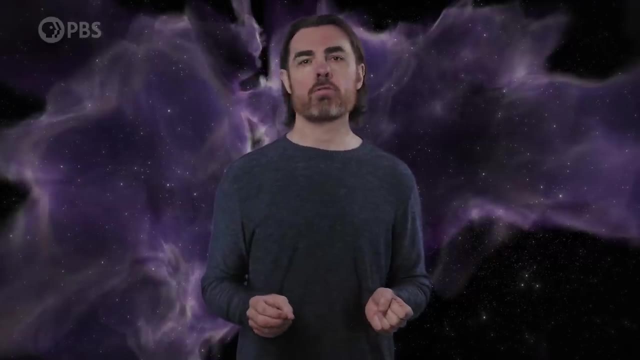 down and at different rates. But by measuring the rate and timing of anti-hydrogen atoms that reach both the top and the bottom of the chamber compared to regular hydrogen, the relative gravitational acceleration on the atoms can be calculated And after the first run of the Alpha G experiment it turns out that acceleration 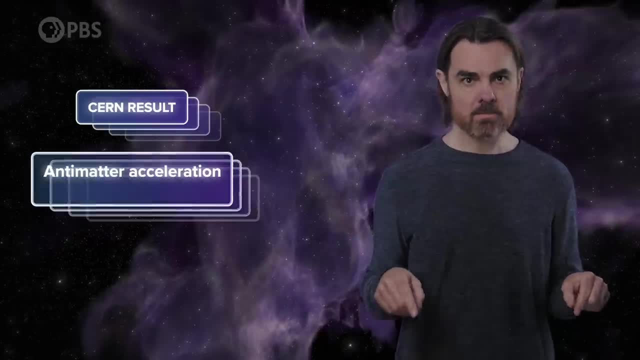 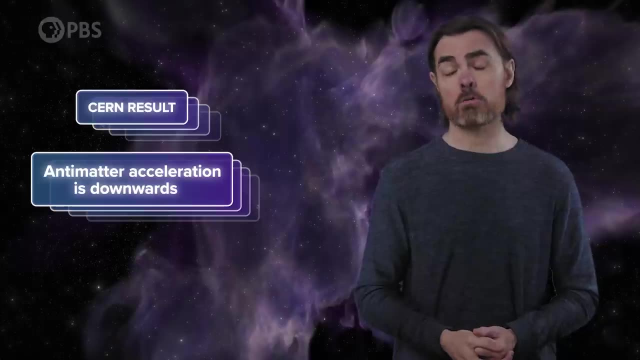 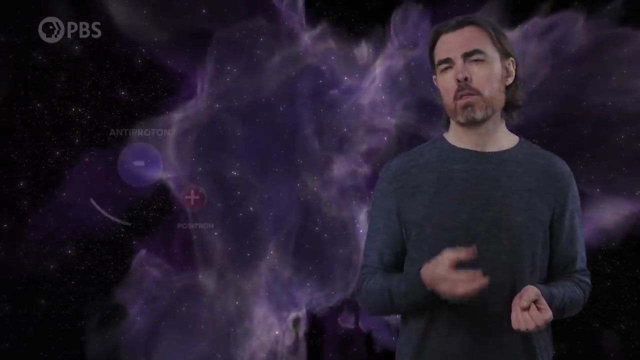 isdownwards. Yep, they're almost certainly not falling up, and that likely dashes our hopes for repulsive gravity from antimatter. However, there is tentative evidence for something interesting: The gravitational force may be slightly weaker on these anti-hydrogen atoms. compared to regular hydrogen. This fairly preliminary data suggests that the gravitational acceleration on the anti-hydrogen is 0.75 ± 0.13 times that of regular hydrogen atoms, meaning antimatter might fall a bit slower. That actually sounds like a big difference, but it's less than. 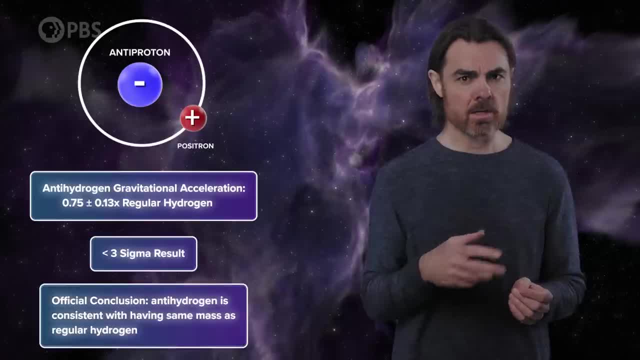 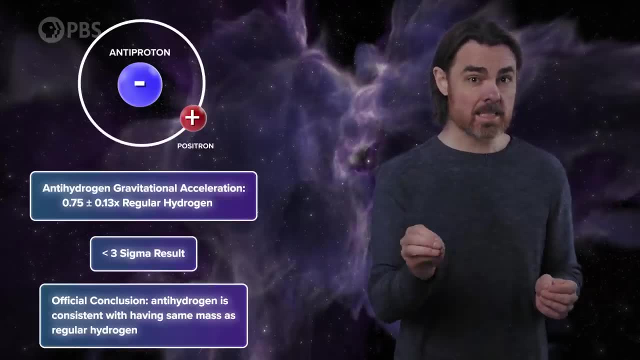 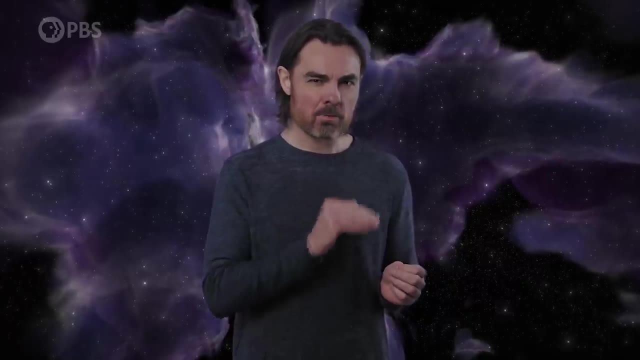 a 3-sigma result, so it could be a fluke. In fact, the scientists of the Alpha G paper do claim that the gravitational acceleration of antimatter is consistent, with it being the same as regular matter, And that's because misleading sub-3-sigma results happen all the time, And when it's. 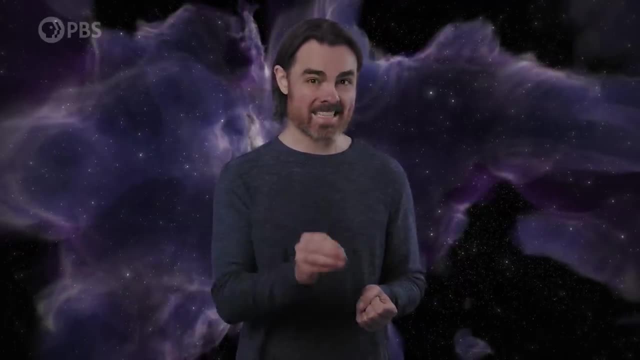 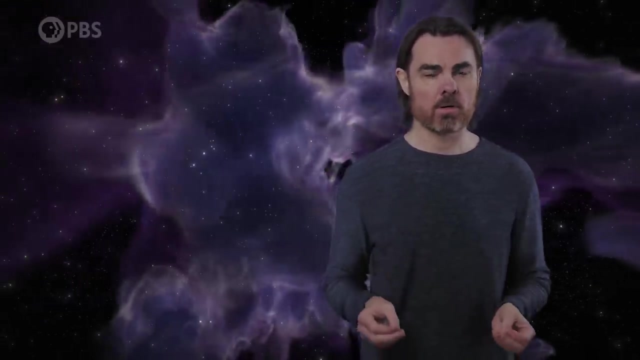 something really unexpected like this, it's much more likely to be a statistical fluke. Remember, we're dealing with only hundreds of atoms here, so random variation is going to be significant. That said, if there is a difference in the gravitational force felt by matter versus, 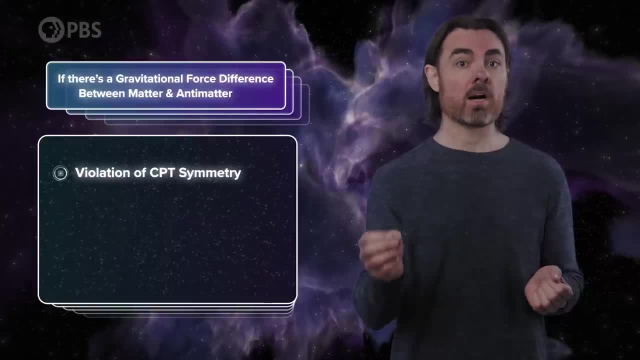 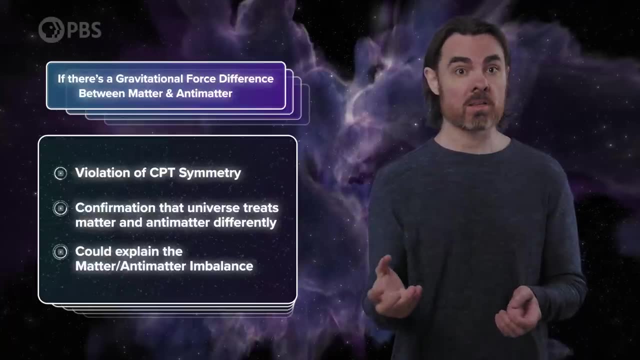 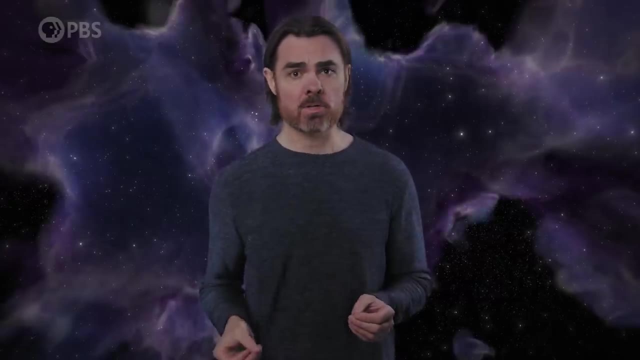 antimatter. it would be extremely exciting. It would mean a violation of CPT symmetry. it would mean the universe treats antimatter differently to regular matter, perhaps explaining why there's this enormous imbalance between the quantities of each. Alpha will continue to build anti-hydrogen atoms and Alpha G will continue to drop them. 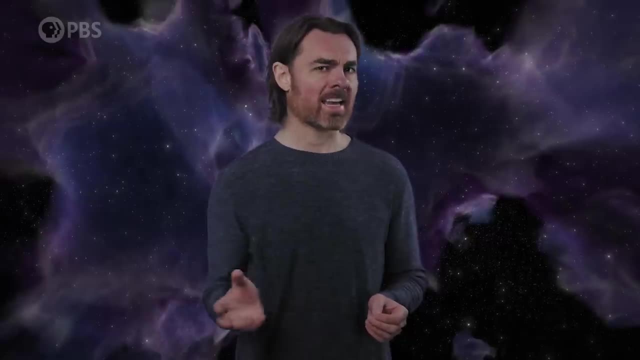 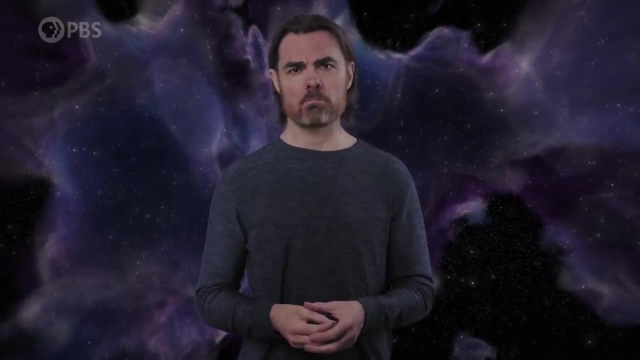 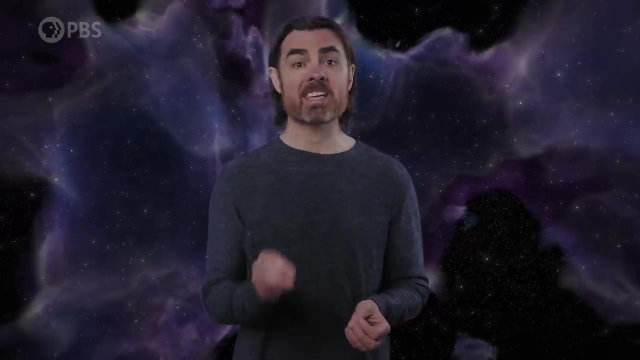 and they will fall down, but whether they fall at the same rate as regular hydrogen will be known with increasing confidence over the next few years. So we may not have a clear path to our levitating cars, at least yet, but we do have a path to either solidifying or breaking. CPT symmetry or either breaking it, So we may have a path to either solidifying or breaking CPT symmetry, or either breaking it, So we may have a path to either solidifying or breaking it, So we may have a path to either solidifying or breaking it. 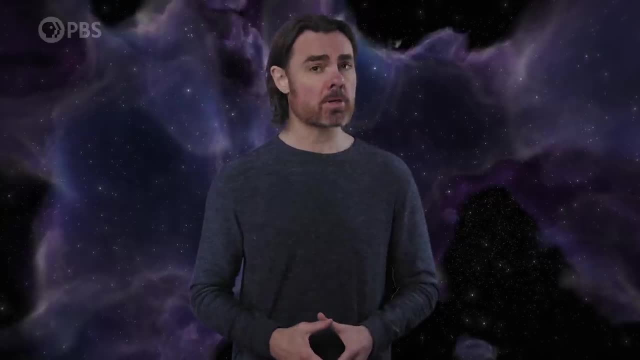 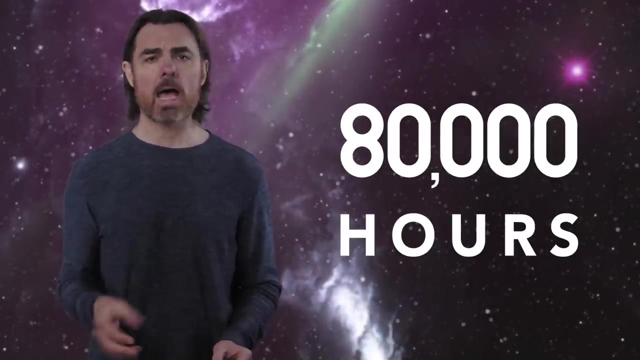 And so understanding what's currently the most fundamental symmetry in space-time. Thank you to 80,000 Hours, a project of Effective Ventures for supporting PBS. 80,000 Hours is a non-profit that aims to help people have a positive impact with their career. 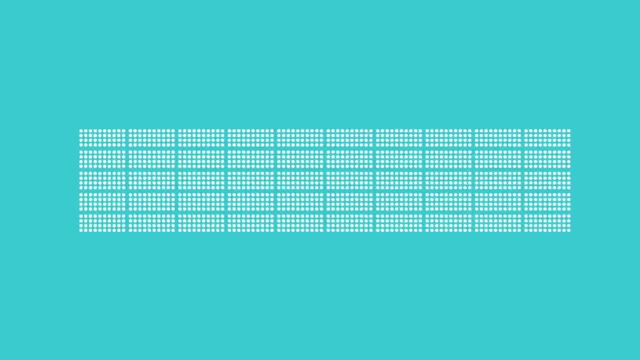 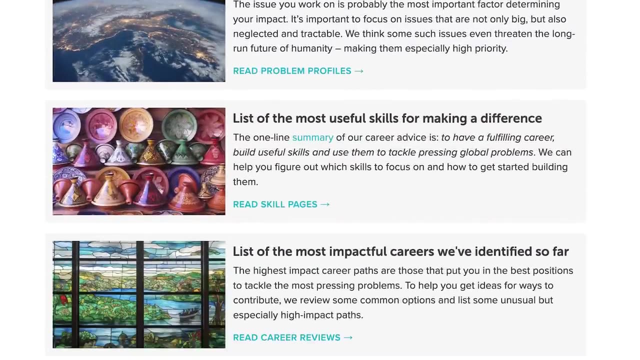 In an average career, you'll work 40 hours a week, 50 weeks a year. for 40 years That adds up to 80,000 hours, And how you spend that time is a very important decision for you and the impact you can.